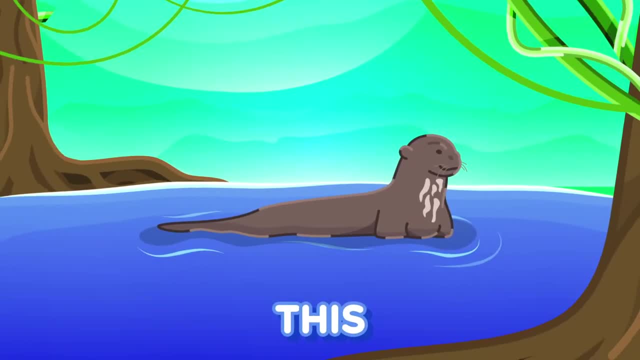 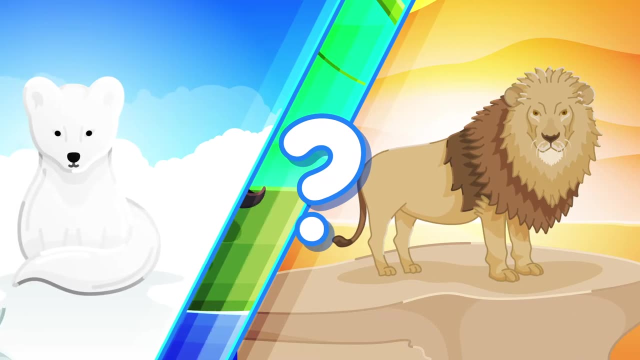 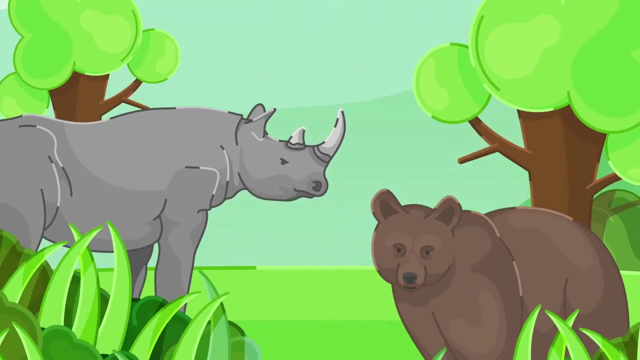 This is an alligator snapping turtle and this is a giant otter. But what do these two creatures have in common with a lion and an arctic fox? Believe it or not, these animals are equal on the food chain, From the biggest mammals to the tallest trees, all the way down to the smallest. 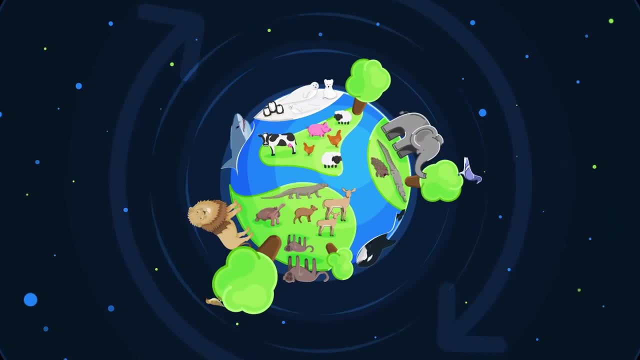 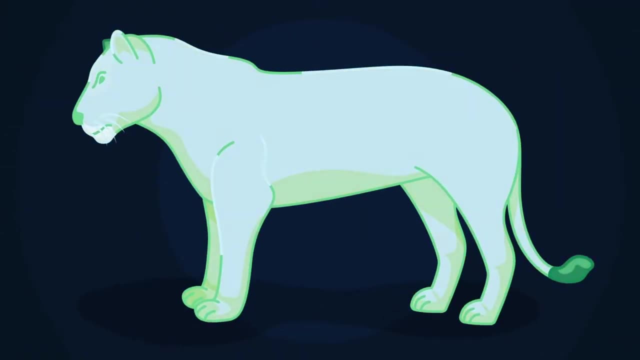 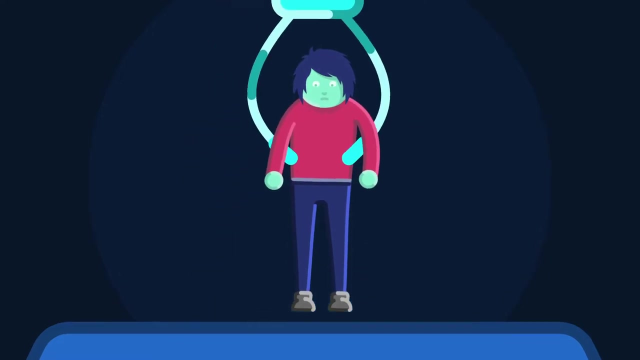 creatures- Everything living on planet earth- needs energy to survive. The food chain is the transfer of energy from one organism to another until it reaches the top of the chain. You might think that humans are the clear favorite to be at the top. However, on a scientific level, we're low in the ranks Somewhere between pigs and plants, Whilst our ancestors used to be apex predators. since the stone age and the development of tools allowing us to consume what is now around 80% of our diet as plants, We've fallen down the ranks, But out of all the apex predators from around the globe. 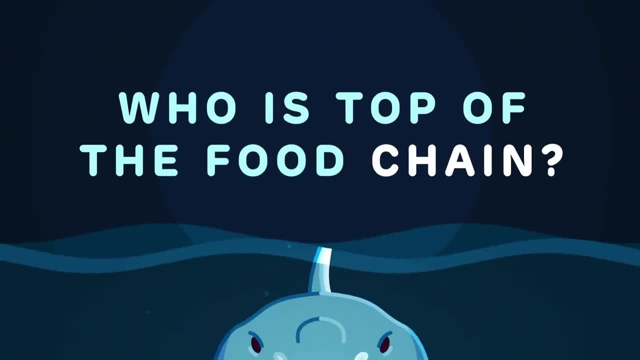 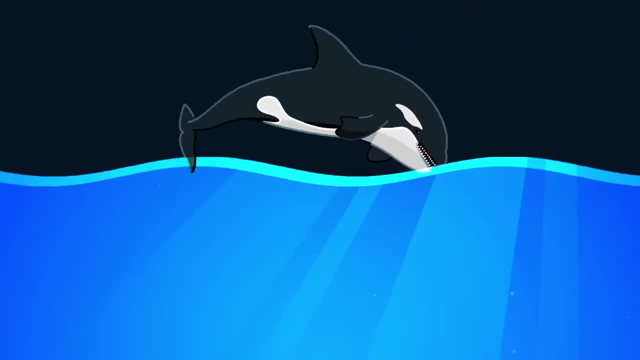 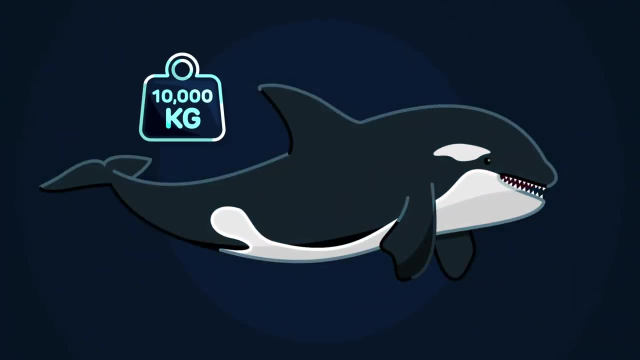 who is top of the food chain. While great white sharks may be what comes to mind when you think of the king of our oceans. the orca, otherwise known as the killer whale, is the true ruler of our waters, Weighing up to 10,000 kilograms, with a dorsal fin up to two meters high. these ocean, 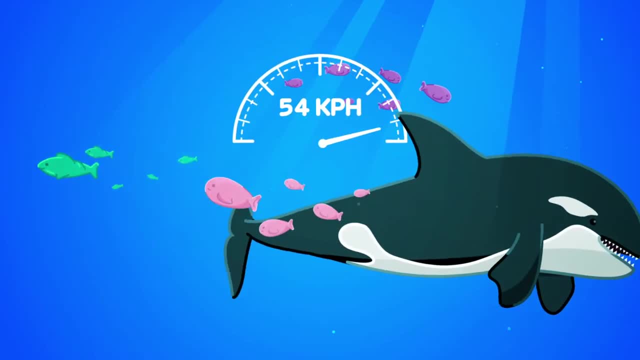 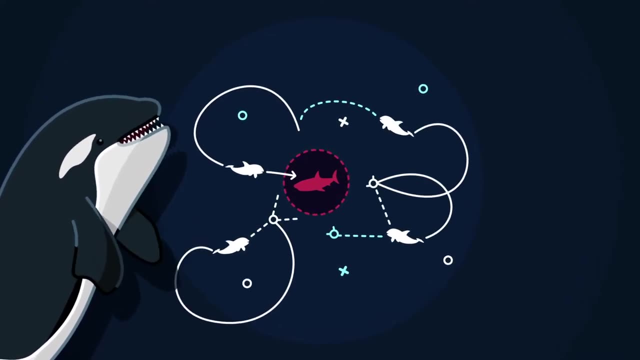 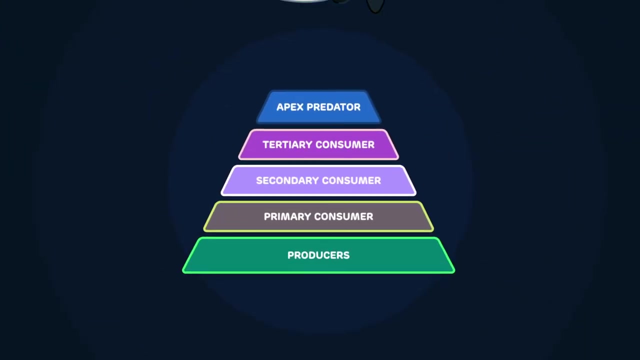 dwellers can swim up to 54 kilometers per hour. Known to be highly intelligent, these whales use tactics working together in pods to take down their prey. They're even known to attack the great white shark. Whilst orcas are the clear winners in our oceans. to discover the top inland predator isn't 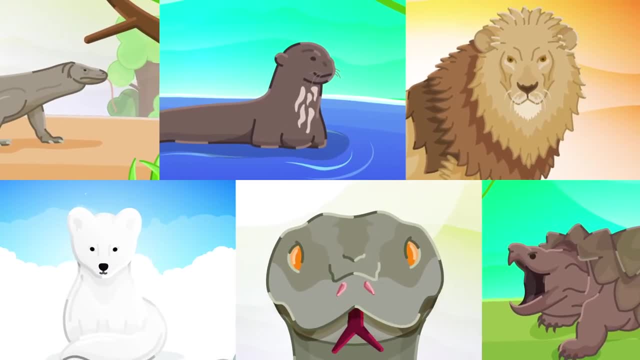 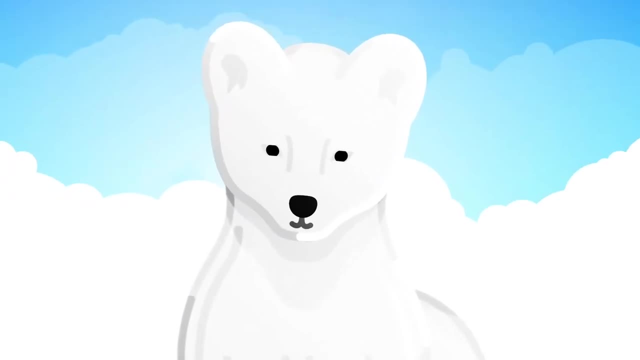 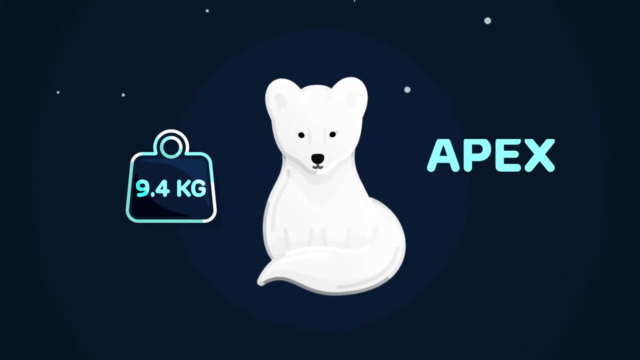 so simple. Many animals live at the top of the food chain, ruling their own kingdoms, as they have no predators in their natural habitats. In Svalbard, this arctic fox, weighing up to only 9.4 kilograms, is an apex terrestrial predator as it lives in such a remote location. 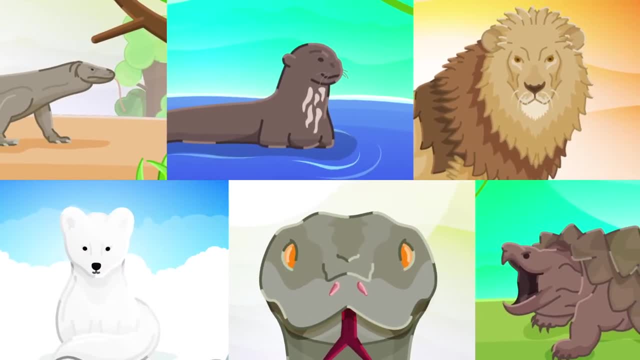 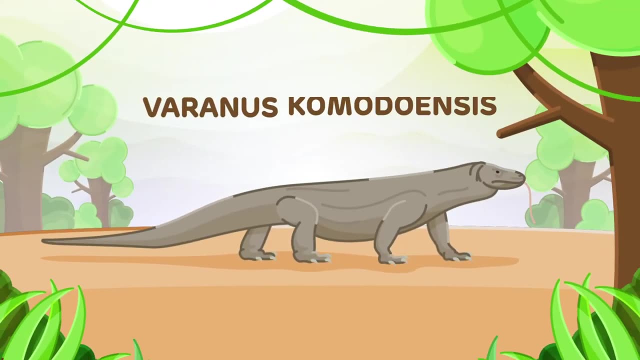 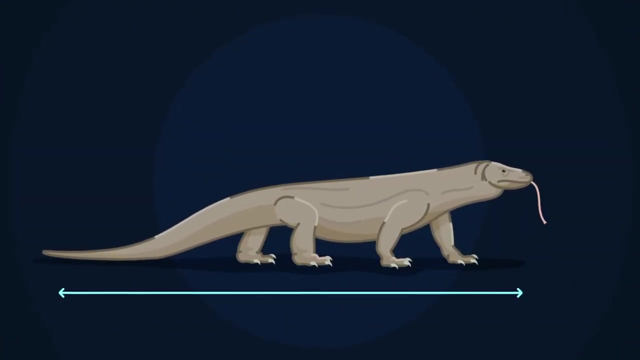 But let's take a look at some of the more deadly species of animal on Earth Living in southeastern Indonesia. the Varanus commodiensis, more commonly known as the Comodo dragon, is the largest lizard on this planet, measuring up to an incredible three meters in. 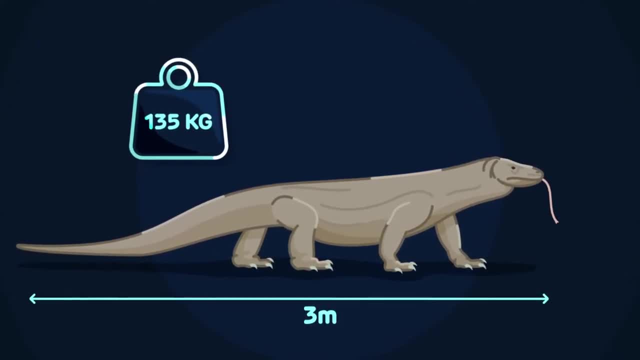 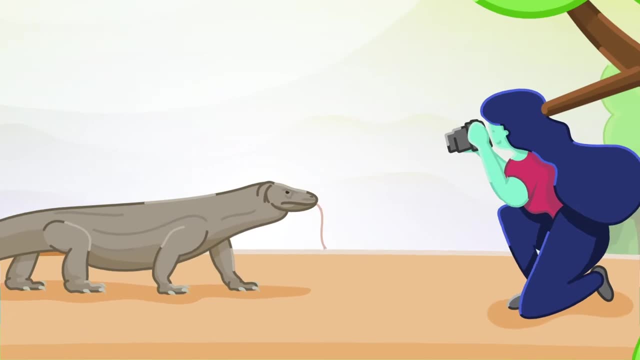 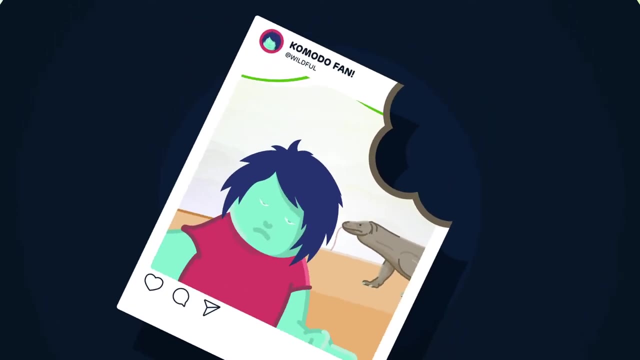 length and weighing up to 135 kilograms. This giant reptile has been popularized through ecotourism due to its incredible size. But don't be fooled by pictures on Instagram. this creature is deadly Fast and ferocious. it is known to hunt anything in sight, including pigs. 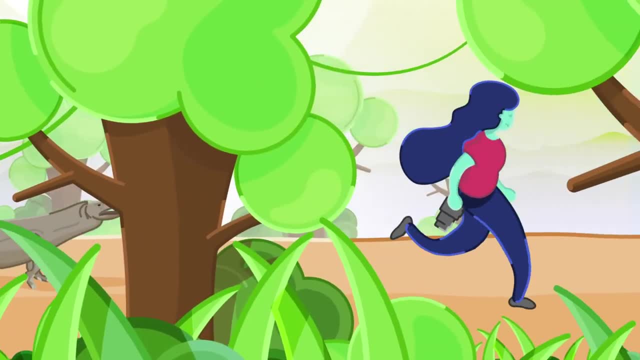 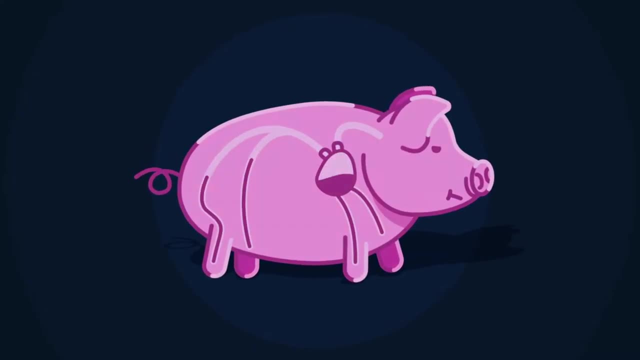 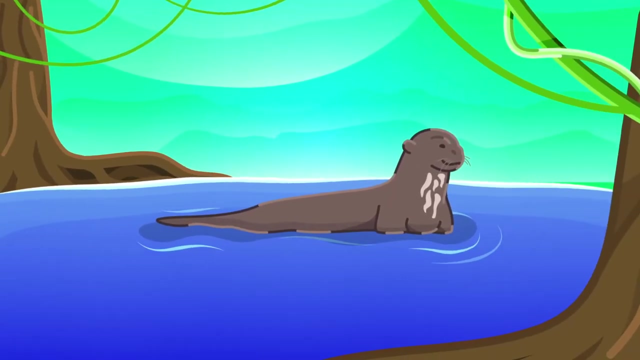 deer water buffalo and even attacking humans With a venomous bite, it causes its prey's blood pressure to rapidly decrease, rendering the animal too weak to fight back The giant otter. Whilst this semi-aquatic creature might look cute and innocent, 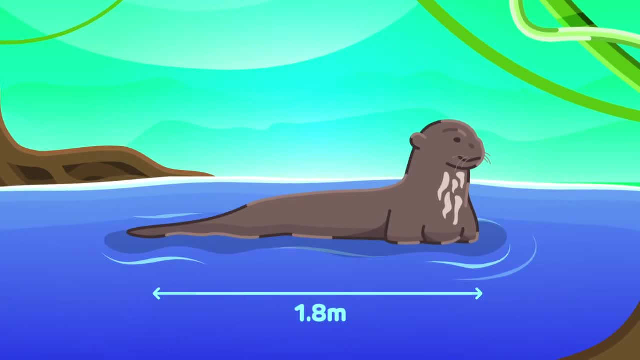 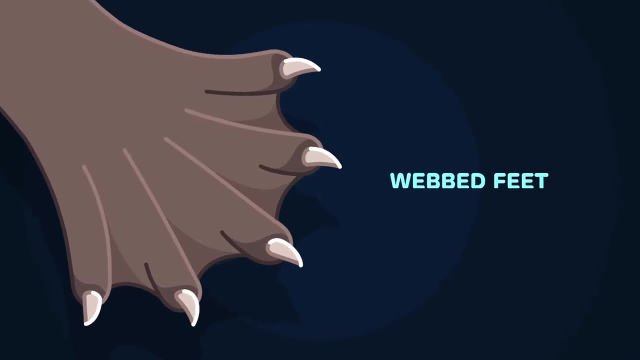 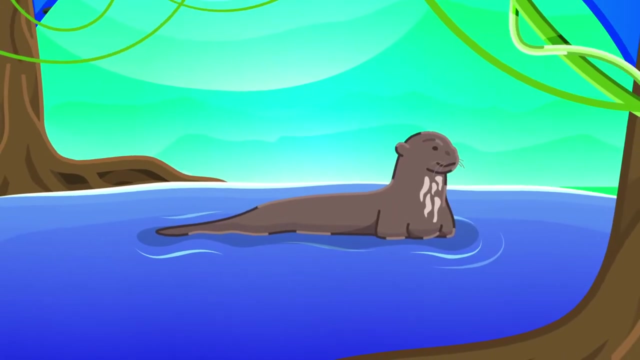 this otter is 1.8 meters long and dominates the river creeks of the Amazon. With webbed feet, made for speed, but also armed with sharp claws, it uses its muscular tail to propel itself through the water. Living in families of up to 20, these cute but mighty animals, 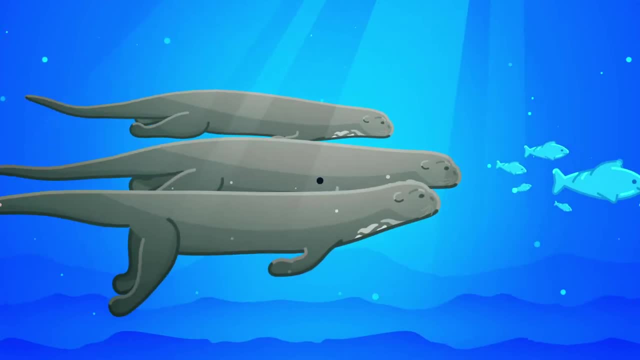 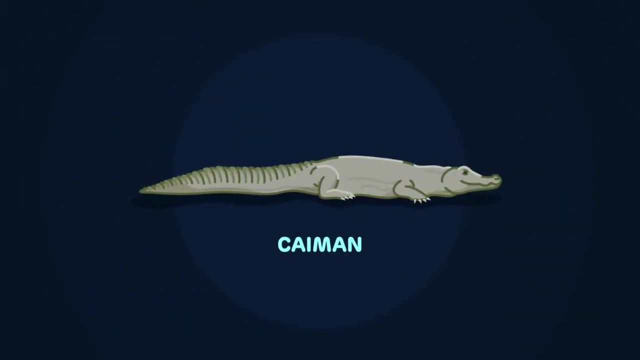 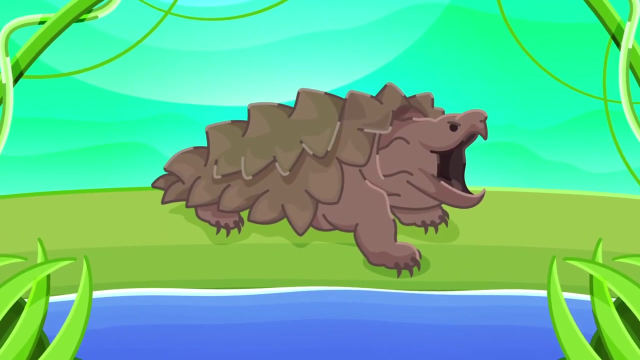 work both alone and together to take down their prey, which includes everything in sight, from fish through to anacondas and even caiman Native to freshwater ecosystems in North America. the alligator snapping turtle is the most dangerous turtle on planet Earth, With ancestors. 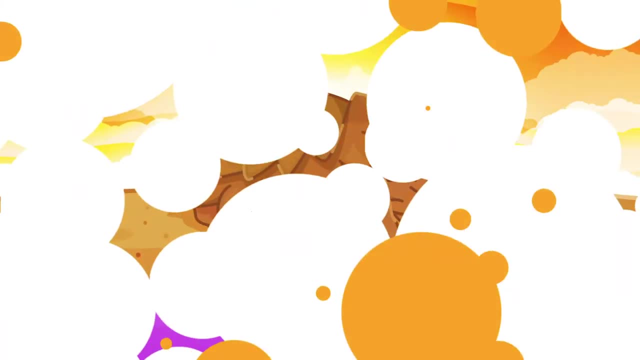 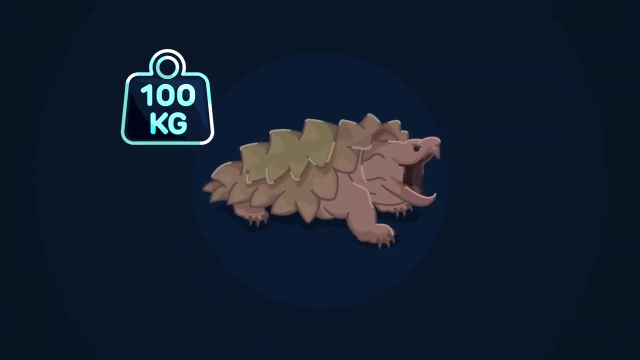 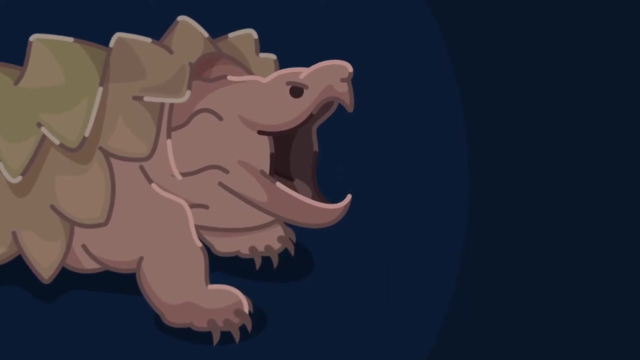 that survived the asteroid that eliminated the dinosaurs. this species has a resilience like no other. Weighing up to 100 kilograms and standing up to 80 centimeters in length, this animal has a jaw that can bite through bone with ease, Utilizing stealth hunting tactics. it 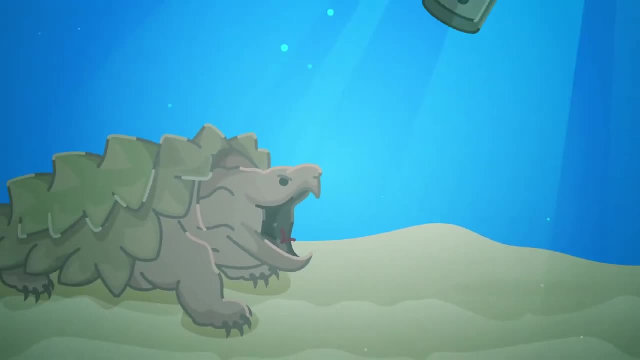 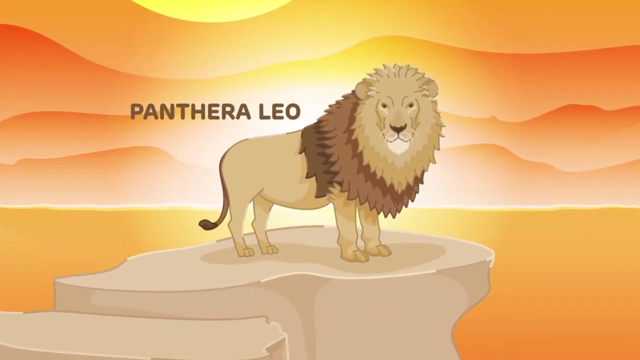 uses its tail to propel itself through the water. The alligator snapping turtle is the most dangerous animal. It uses its tongue to lure its prey into its mouth and can stay underwater for up to an hour at a time. The panther aliyah, otherwise known as the African lion, is the king of sub-Saharan Africa. 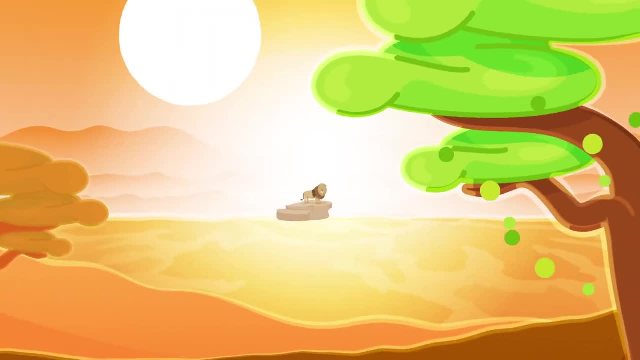 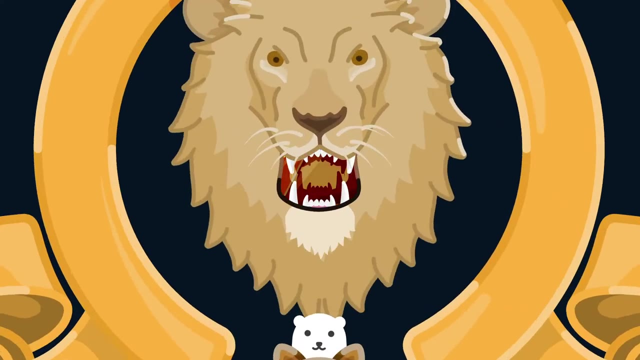 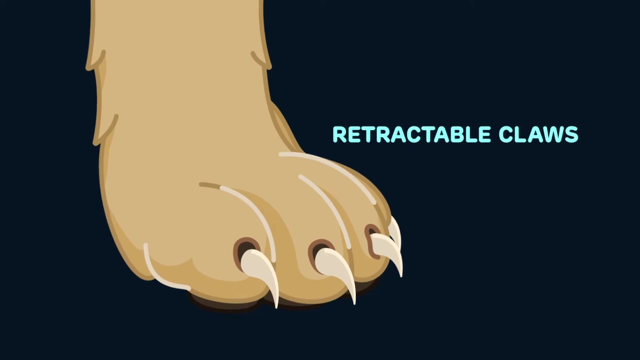 With a roar so loud that it could be heard up to 8 kilometers away. these iconic creatures were seen as a symbol of power and strength all the way back to ancient Egypt. Using paws with razor sharp, retractable claws, along with their mighty jaws lined with large fangs, they outperform all. 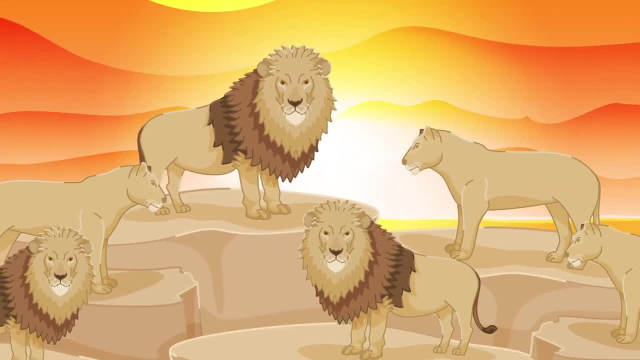 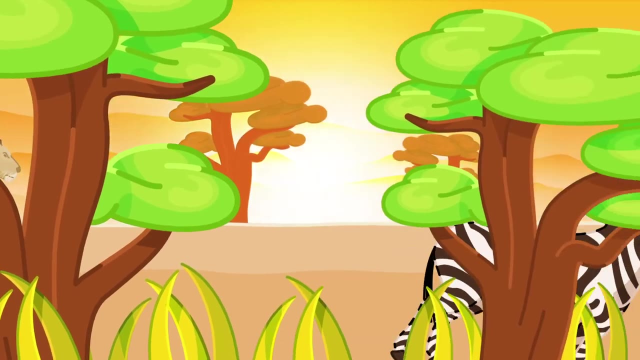 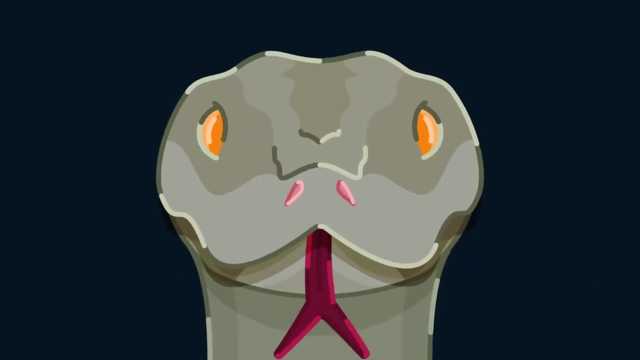 who stand in their way. Living in prides of up to 40, female lions take the lead, working together to hunt large prey, including zebras, buffalo, and are even known to attack giraffes. The Burmese python, one of the largest snakes on earth, growing up to an incredible seven meters in length, and 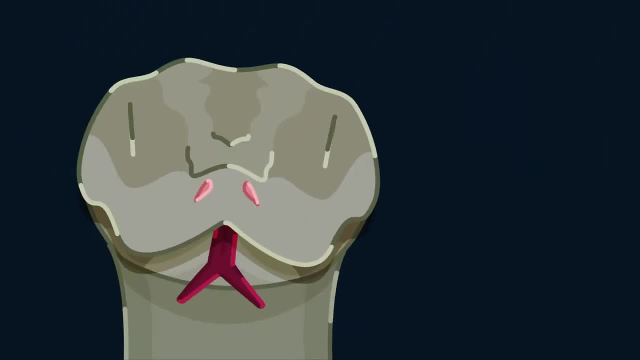 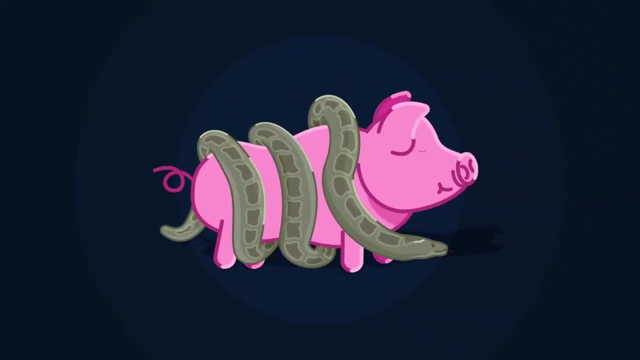 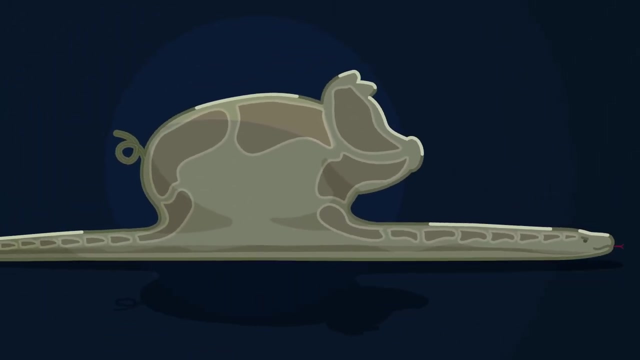 weighing up to 90 kilograms. These cold-blooded reptiles are non-venomous. instead, they wrap around their prey and squeeze them with ever increasing pressure. Due to their enormous size, they're even known to consume their prey whole. Although native to Southeast Asia, in August, 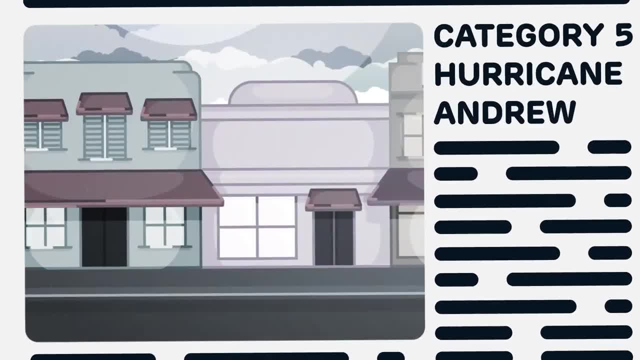 North America. the Burmese python is the largest snake on earth. The Burmese python is the largest snake on earth. it was once considered the largest snake in the world. It was an annual human species during the late 1990s. In 1992, category 5 hurricane Andrew hit florida, leaving a spate of destruction in its path. One of the buildings affected was a python breeding facility, which became a catalyst to the Burmese python breeding in the Florida Everglades. This population has continued to grow and now stands between 30 000 to 300 000.. But what about the greatest apex predators? 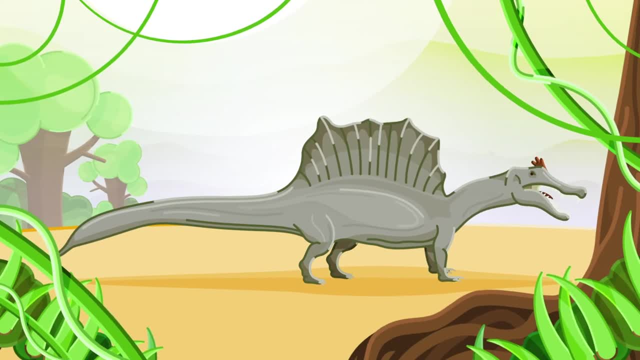 to be нашed and secured and traveled. The Burmese python. a few years of the Burmese python is the most of all time. The Spinosaurus lived around 100 million years ago and is believed to be one of. 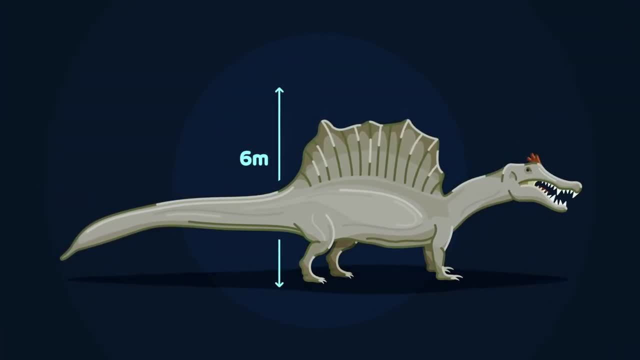 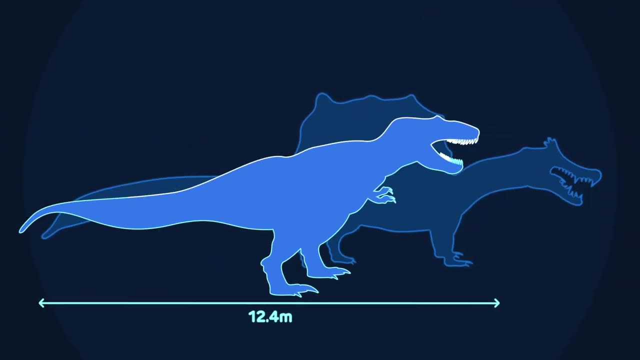 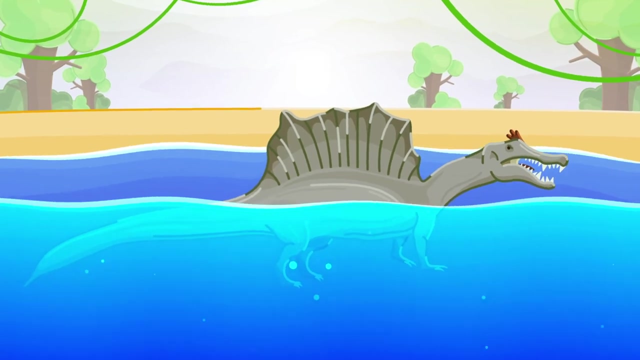 the greatest ever, Standing up to 6 meters tall and 15 meters in length. this creature was bigger than a London bus, Tyrannosaurus rex and even the Giganotosaurus. This ancient dinosaur lived on both water and land, similar to modern day crocodilians, Whilst it had very little predators. 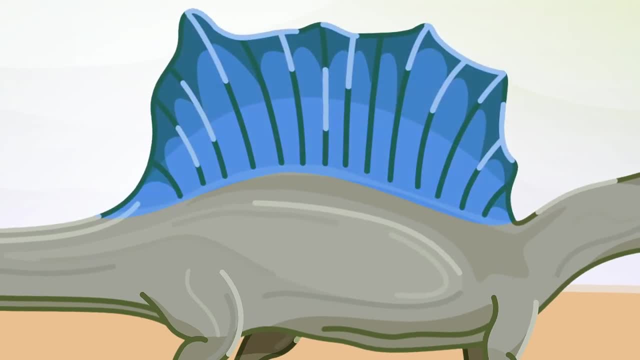 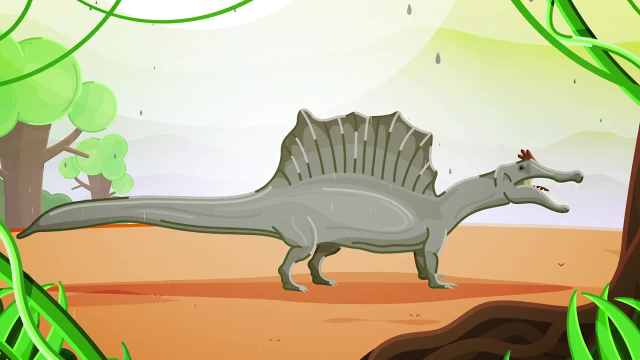 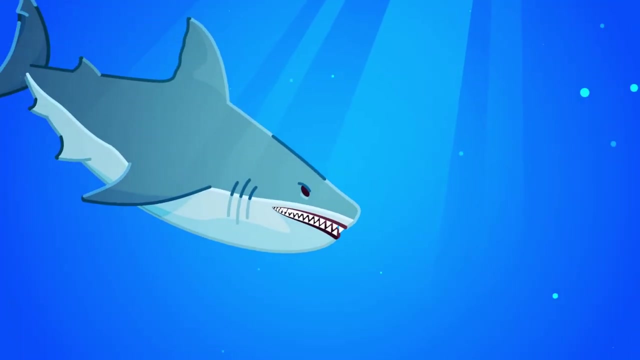 due to its enormous size, it had a sail, which scientists speculate that if these creatures sensed danger, it could expand to make it appear even bigger, to scare away animals and even other Spinosaurus. The Megalodon is another ancient animal deemed one of the greatest predators.